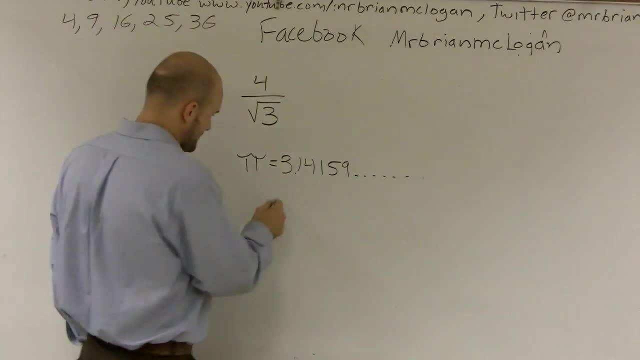 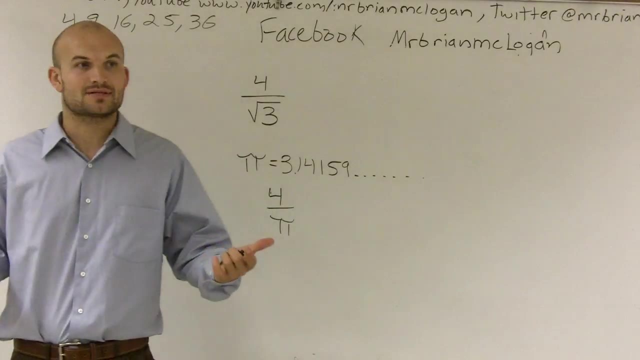 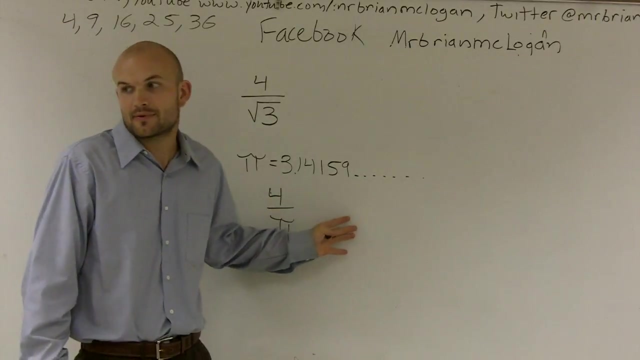 going on and on forever. So if I was to divide, let's say I divided 4, divided by pi, would we ever get a number that stops? Well, no, because since pi never stops, we're never, ever going to get a number that's going to stop, right. So you can't divide 4, you can't divide into. 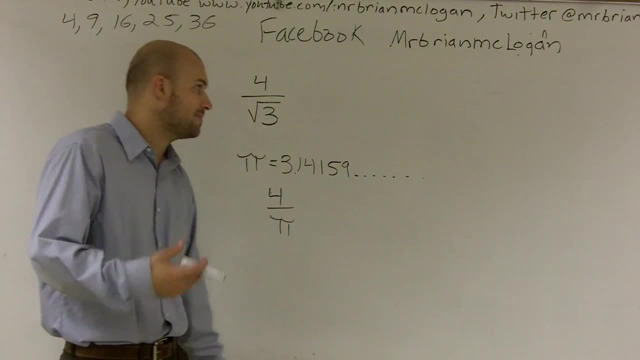 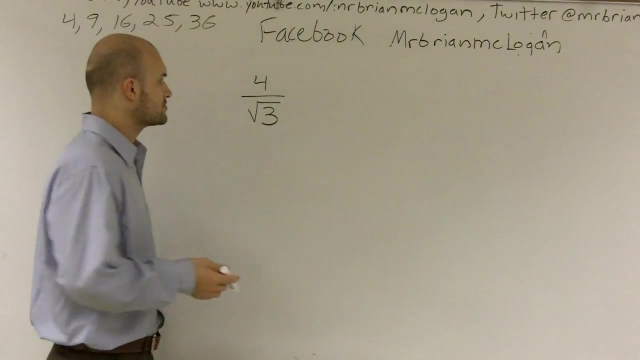 or 4 cannot be divided into pi, or pi cannot be divided into 4.. So we have a little bit of difficulty now simplifying this. However, when you have a radical, a radical has the same properties. This square root of 3 keeps on going on and on and on forever. So it's 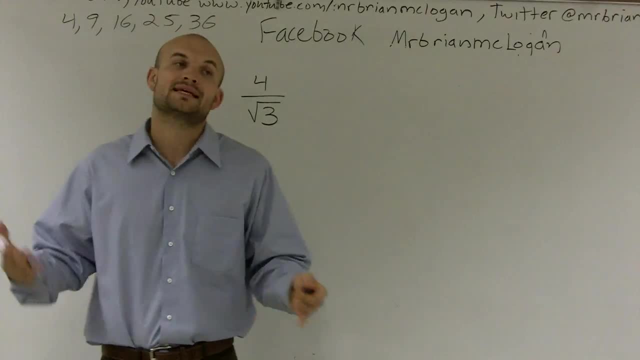 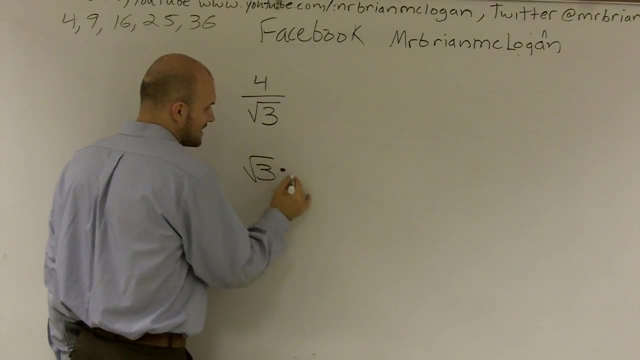 impossible for us to divide this into our 4.. However, what we can do is we can get rid of this radical. And here's what we're going to do: Square root of 3 times the square root of 3.. Whenever you multiply a radical times a radical, you can multiply the two numbers. 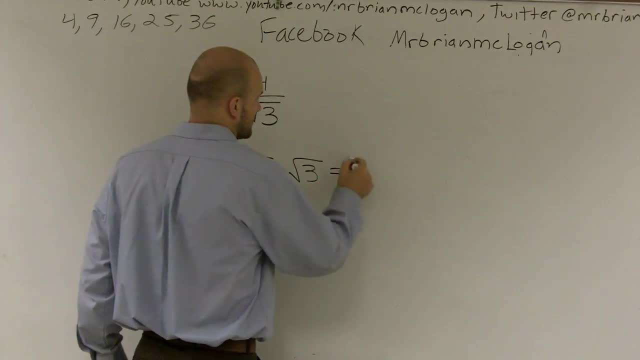 inside the radicands under the same radical. Now we all know that 3 times 3 is 9.. Or I might also just write it like this: all right, Because either way it doesn't matter, This cancels out and that cancels out to give you 3.. Or the square root of 9 cancels out to give. 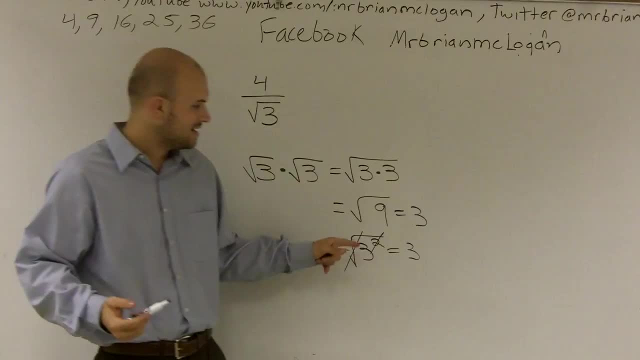 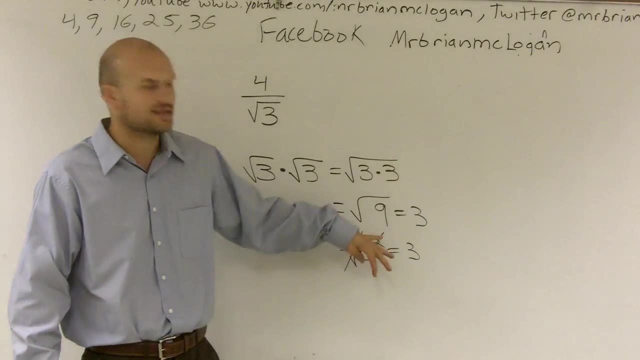 you, 9 equals 3.. So there's multiple ways. I just want to show you this because a lot of times you won't get a square number And you might have to do like the square root of x or the square root of x squared. So you should know that the square root and something 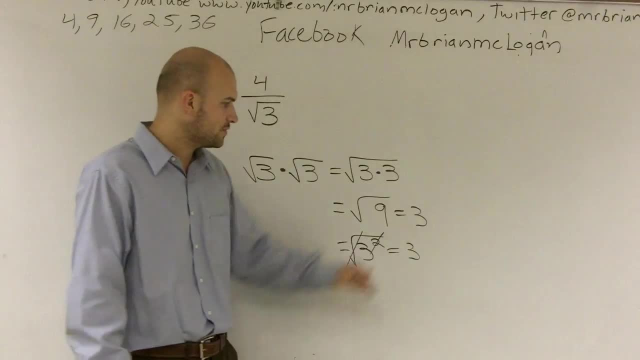 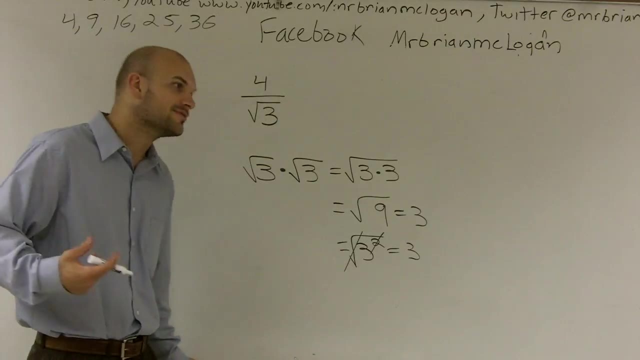 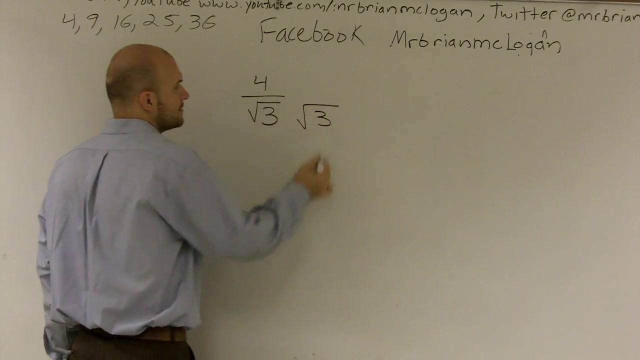 squared are inverse operations of each other, So they cancel out, to give you your radicand. So, if I know, if I multiply this by the square root of 3, I'll get to 3.. Well, that's what I'm going to do. So I multiply by the square root of 3.. So I multiply by the square root. 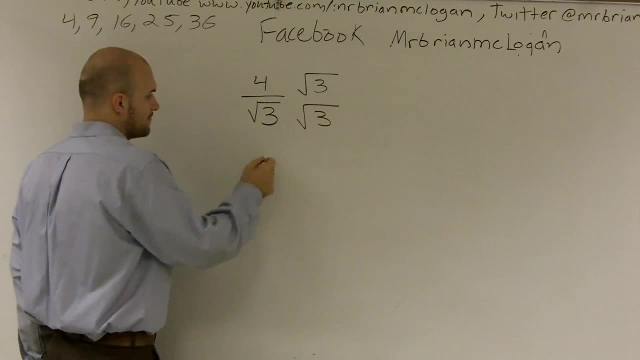 of 3, and I multiply the top by the square root of 3.. Now, why did I multiply the top and the bottom? Well, if I wanted to multiply 1 half times 4,, I'll get 1 eighth, 1 eighth. 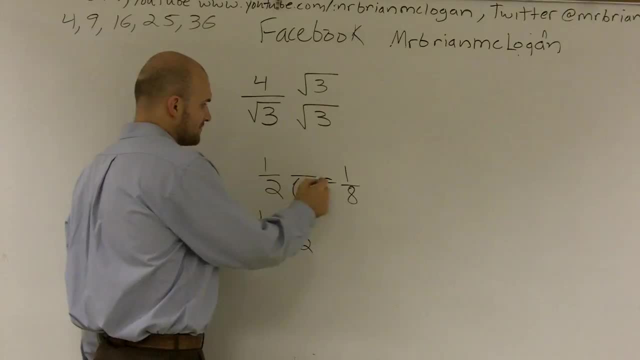 does not equal 1 half, So I want to keep this fraction true. I have to multiply the top and the bottom by 4.. Therefore, 1 half equals 4 eighths. So I'm multiplying, I'm changing the problem.